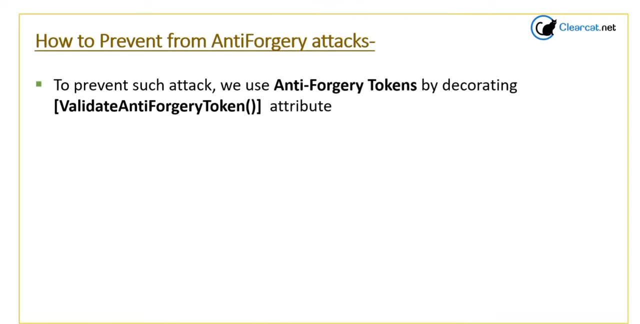 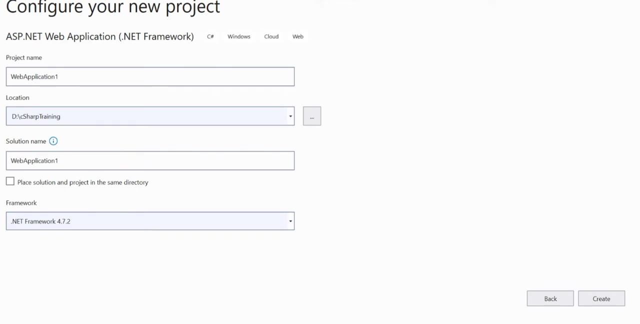 anti-forgery tokens attribute over the method or controller label in MVC or web APIs. So now let's flip over the visual studio and understand the things to code step by step. Okay, so here we are creating a new project which named as anti-forgery token, okay, okay, let's create it and we will choose the MVC project. 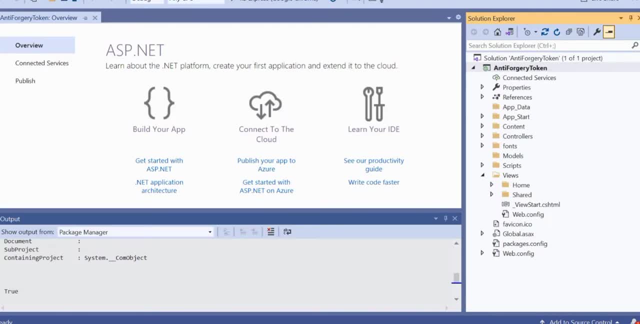 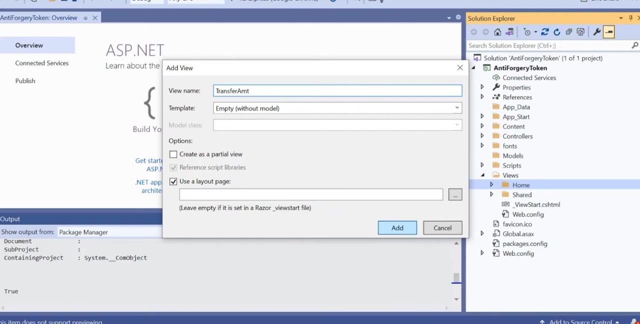 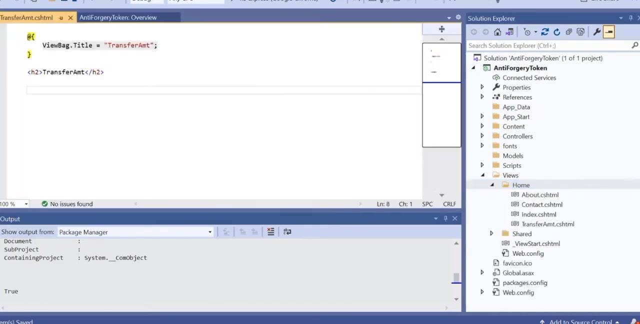 okay, now let's add a new view. So right click on the home and add view. so view name i'm going to provide as transfer amount. okay, let's add this without model. okay, now let's, uh, put some code here, as i already took some piece of the code. in interest of time, 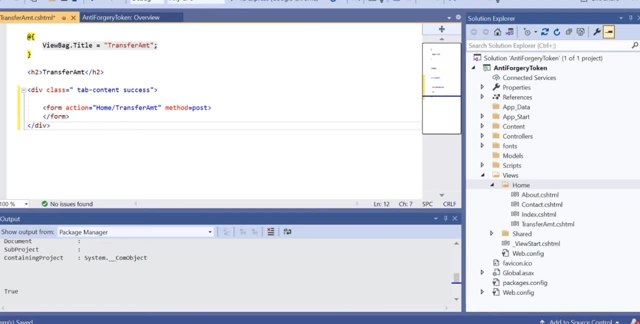 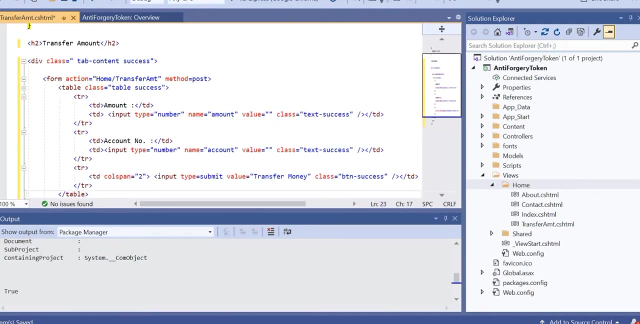 and let's make it transfer amount, Okay, okay. and also let's create here a table inside the form tag, okay, okay. so here we are taking the two input, the first for amount and second for account number, and finally we are submitting this request by the submit button, which is transfer money. so this is what. 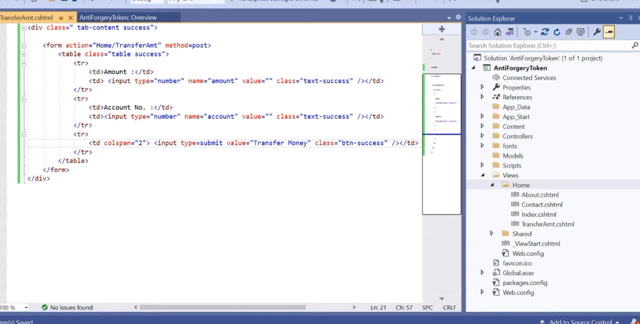 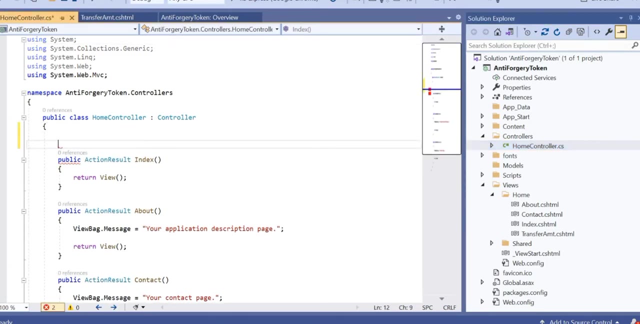 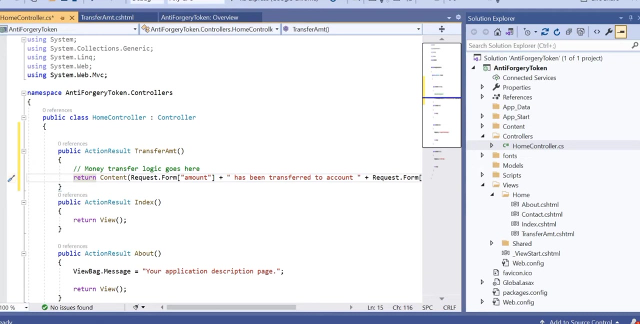 we need to view. all right now let's go to the controller. okay, so inside the controller let's create here the another action result method: public X and result: let's face transfer amount. okay, let's do some code here for the logic. so this the money transfer logic, here we will send. 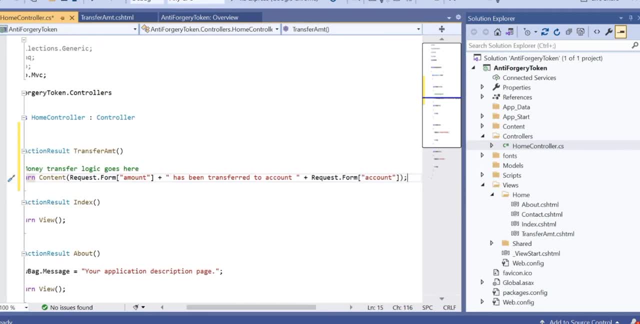 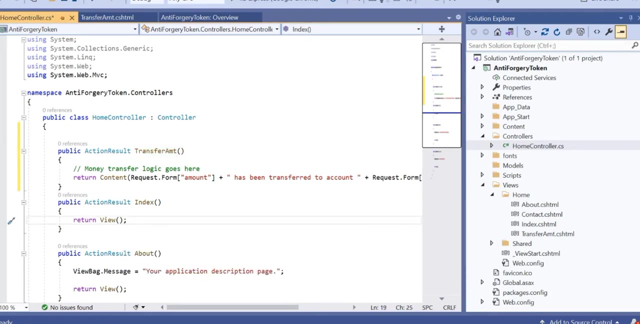 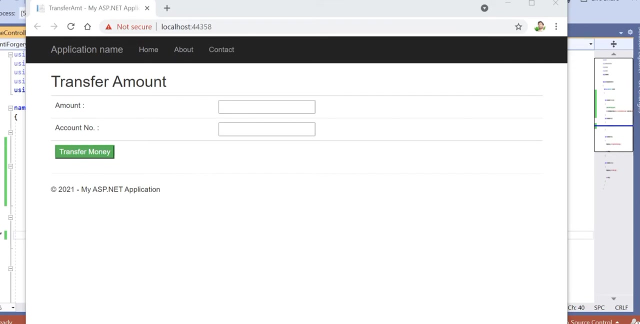 the content after are hitting the submit button that this amount has been transferred to to this account. okay, and let's return this transfer amount view. okay, okay, fine, so now let's run the application. okay, great, so this is what the view looks like. okay, so let's suppose we are going to enter the 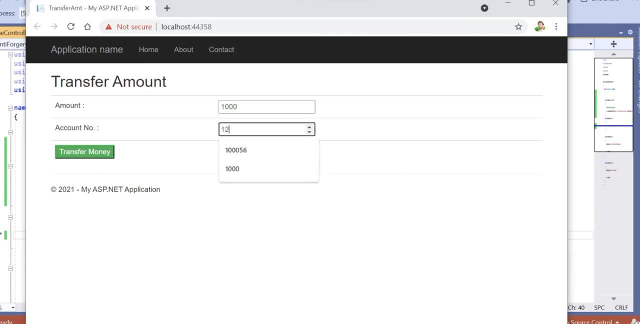 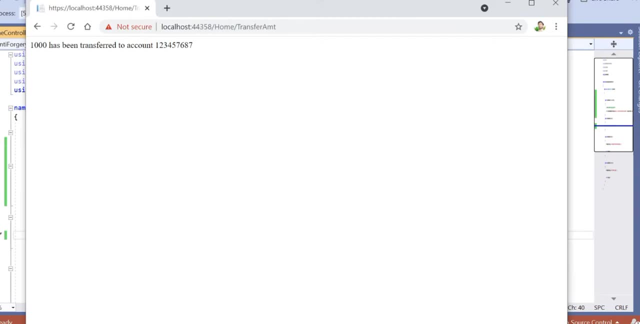 amount, thousand, and account number is one, two, three, five, six, seven, something like that. okay, transfer to money. so what we are getting the content after hitting submit button. thousands has been transferred to account one, two, three, four, five. this is the account number in which we submitted the request. okay. 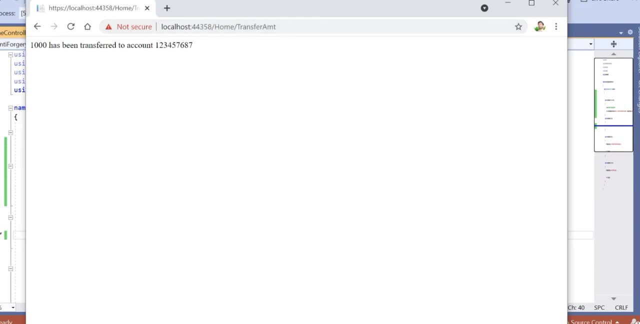 as of now, it works fine, as the authorized user can only can- make the request. but what, uh? anti-forgery comes in scene when uh, the unauthorized user or the malicious user also can, uh can, make the same request by accessing this url from the another sites. let's see how. so let's create another project here. let's give it name. 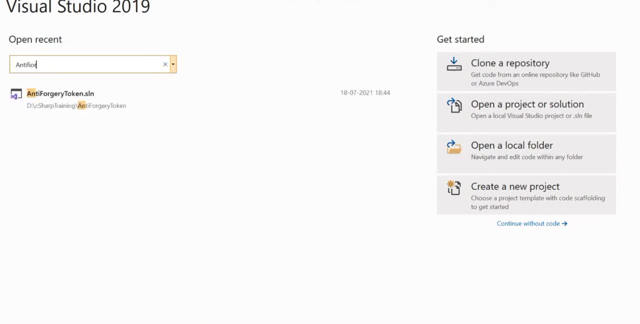 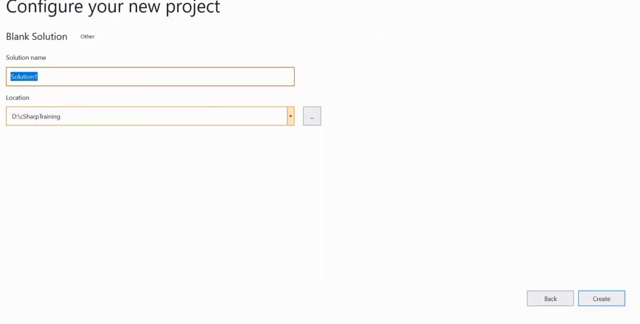 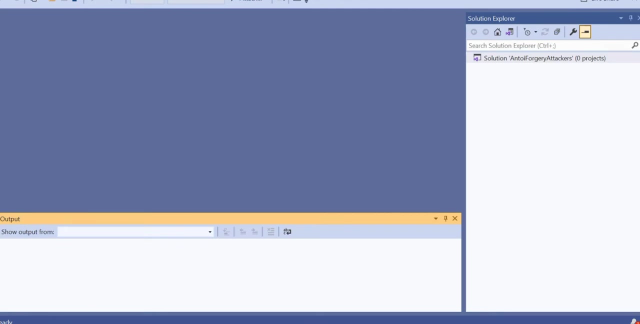 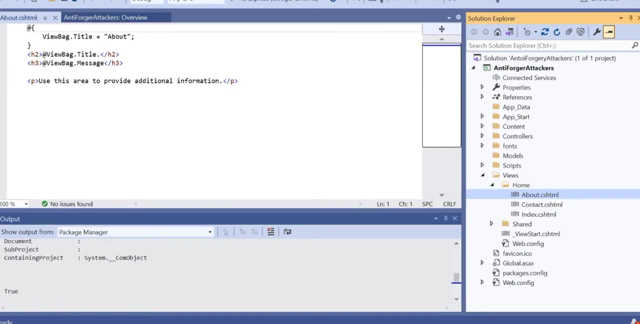 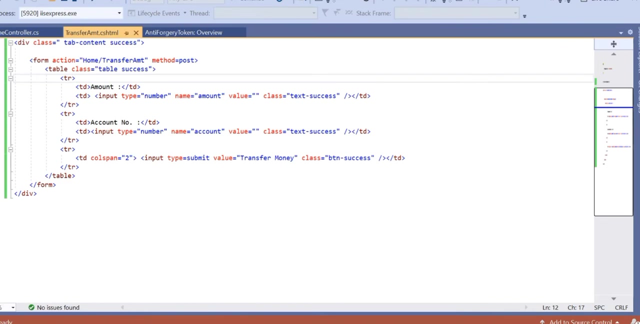 uh, anti forgery attacker. okay, let's create a new project here first. okay, next, anti forgery attackers. let's create here. so we created the new project here. another project: okay, so let's inject some code in about view. okay, so let's take the code from here as well. so i'm taking the complete, this form. okay, so let's take this complete. 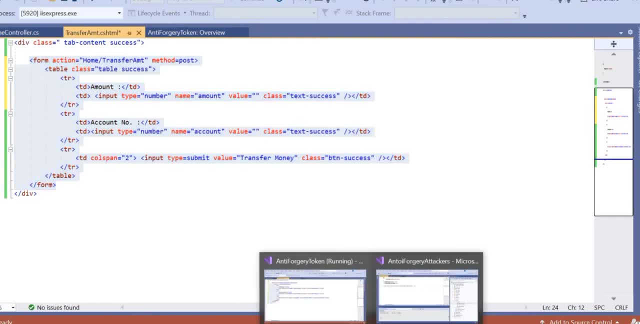 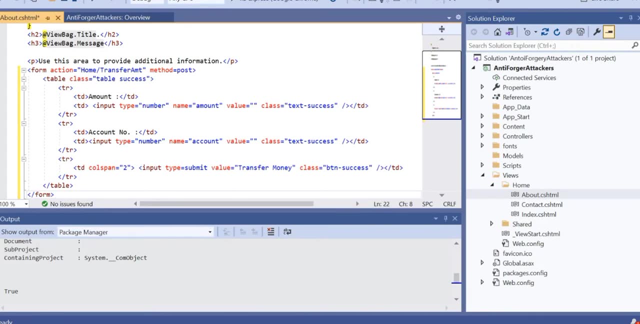 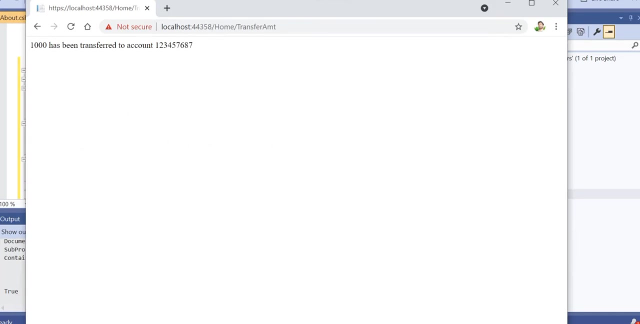 complete form and inject the same code over here. so let's make it attackers page, okay, or we can say here within the h2 tag: okay, fine, and what we need to do here, the action we need to take: the URL of the actual site which is running. so this we want to do, the anti-forgery, we want to send the cross request to this site. 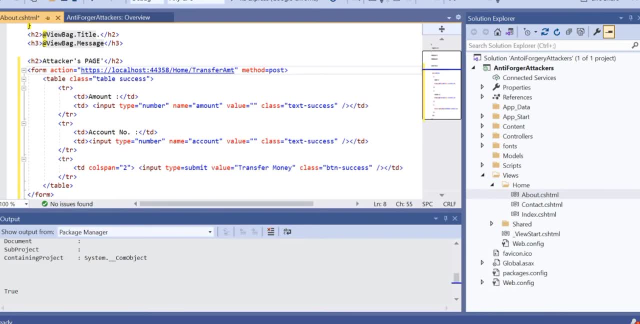 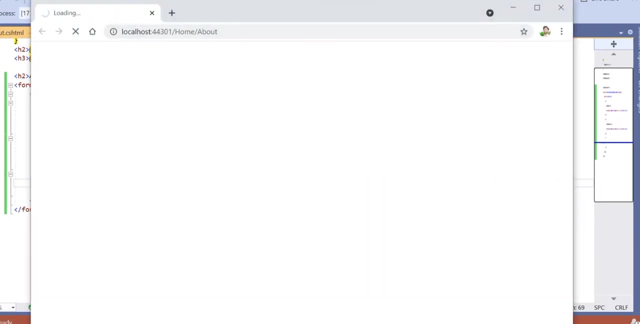 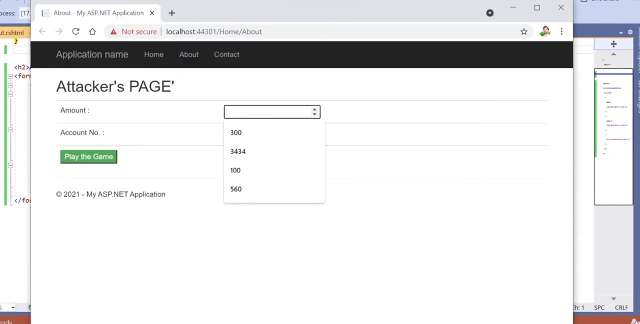 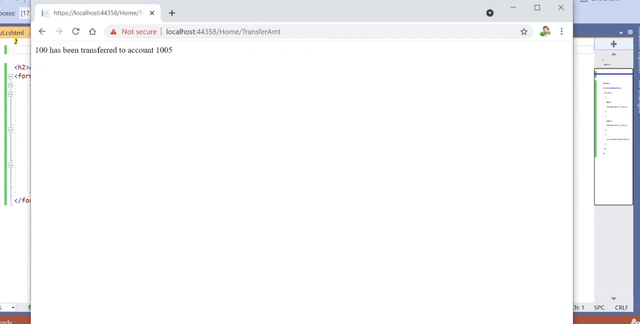 okay. so let's put this here and method will be posted the same. and here let's say: hit, play the game. okay, okay, fine. so now let's run this, you okay. so here let's put some amount, let's say 100, to the account 1005 and let's hit the play the game. 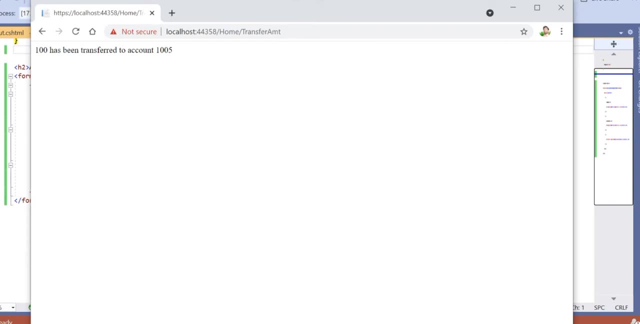 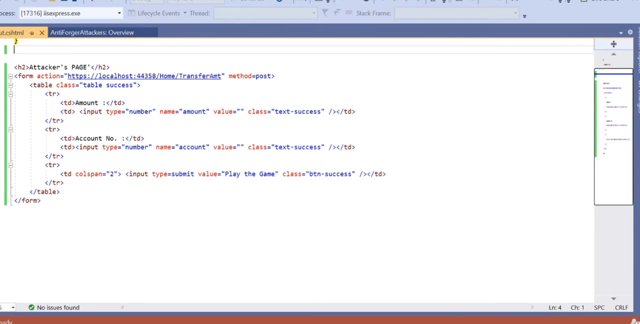 now we can say 100 has been transferred to the account 1005. so what we are doing actually here that we are just uh making the trusted request from here to this URL, which is the actual URL. so this is what uh anyone can do: uh misforgery with your- uh you know- web application and can transfer. 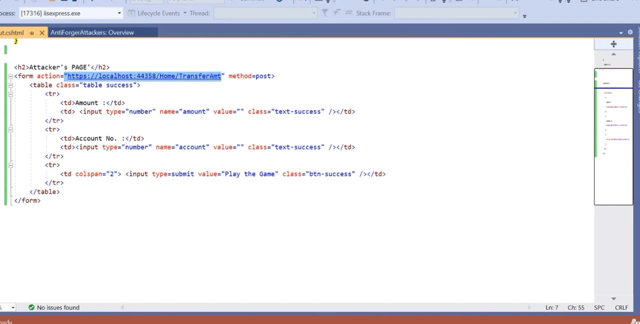 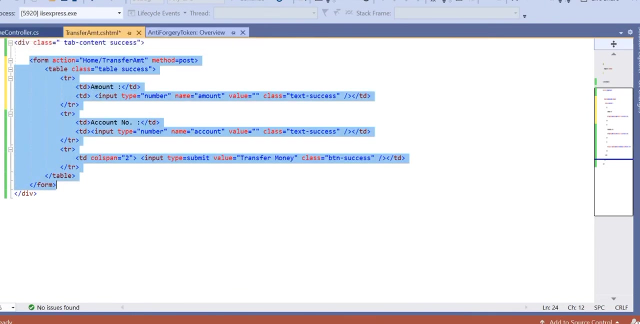 the amount to the account or can do the anything, whatever you are posting the request. so this is what can be attacked by the hackers. okay, in that way. so now thing is that how we can prevent the same. so to prevent the same, let's uh, come into the actual site and here inside the controller. 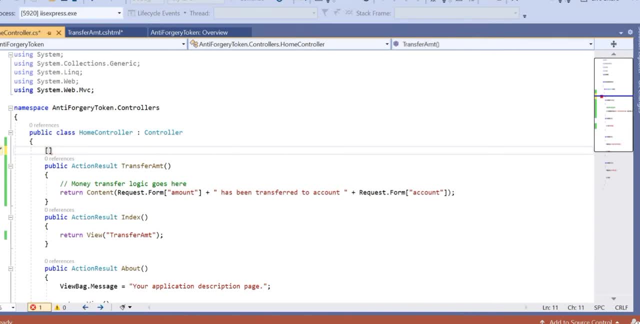 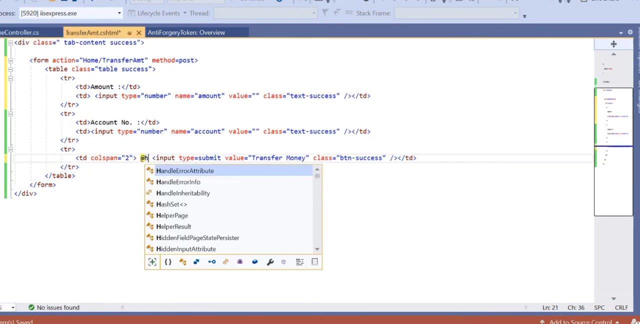 let's uh decorate here validation and t4 forgery token. so if we will do this, so it's not complete things we need to do after this- also, we need to uh take here the at as tml dot anti-forgery token. okay, so now that way, if 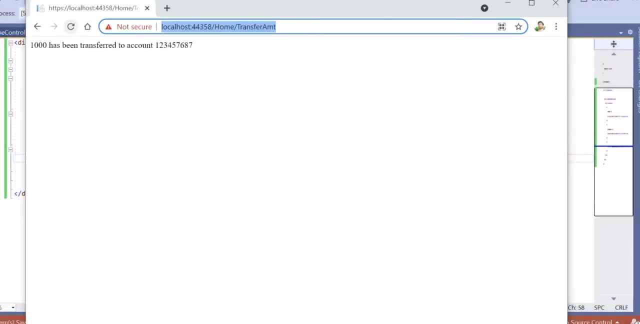 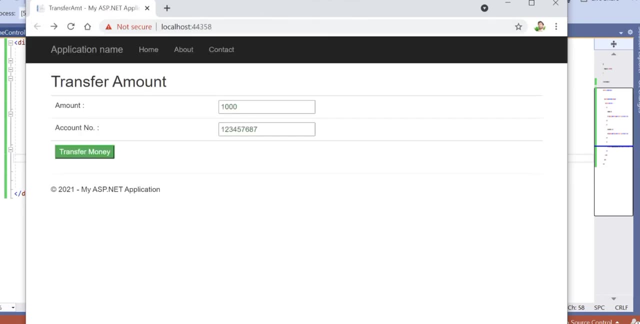 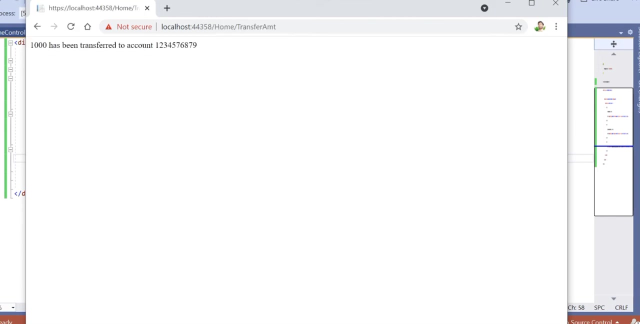 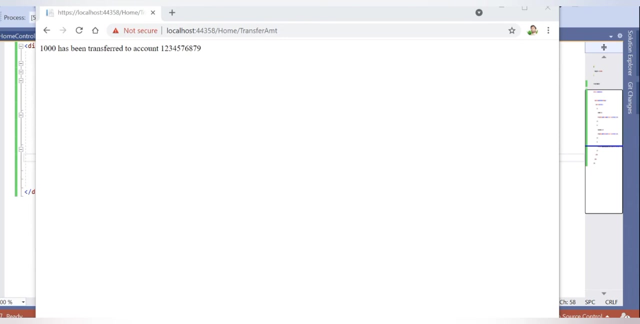 we will uh refresh here. let's see. okay, so it will works fine without any issue, which is our actual site. okay, so let's do here. and let's uh here, do the nine and transfer money. okay, it is working fine. but what will happen now here? okay, so now, uh, let's go to the hacker site from where we are making the request. so this is. 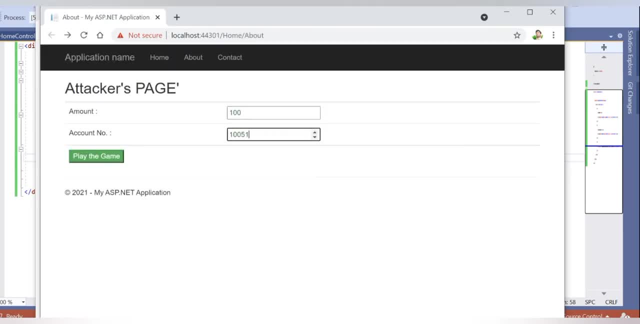 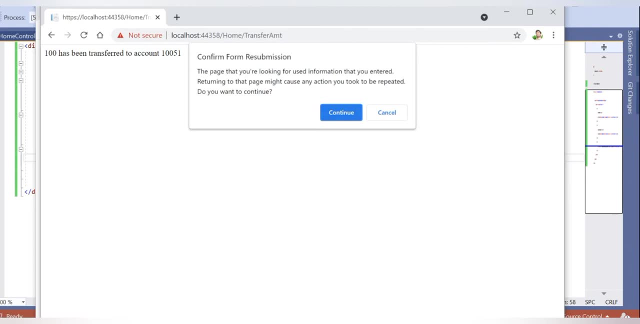 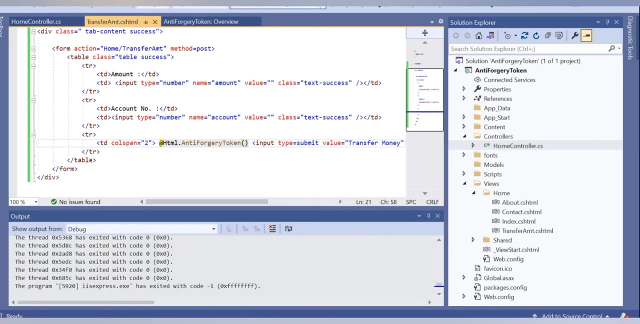 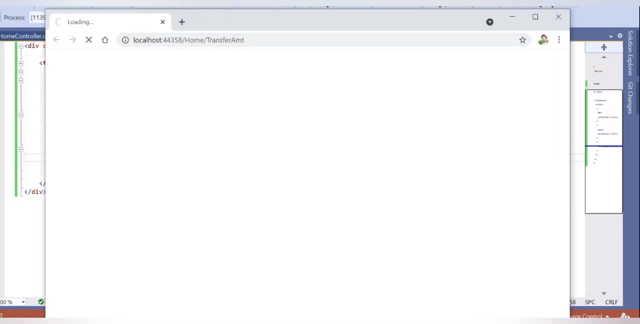 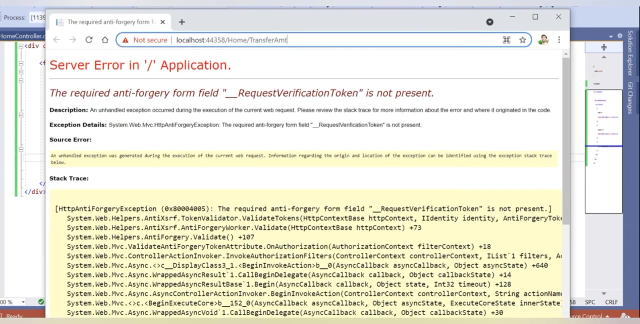 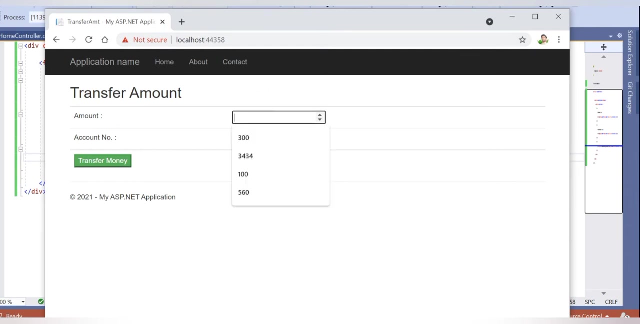 the hacker site. we will see this one right now. let's do here play the game. okay, let's refresh this one as well and let's uh close this here first and then let's run it, okay. meanwhile, uh, okay, see, we have uh to refresh this one, okay, so this is the actual site. so here there is no issue, we can do anything. 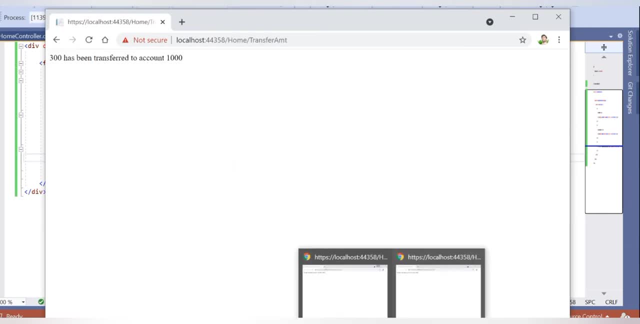 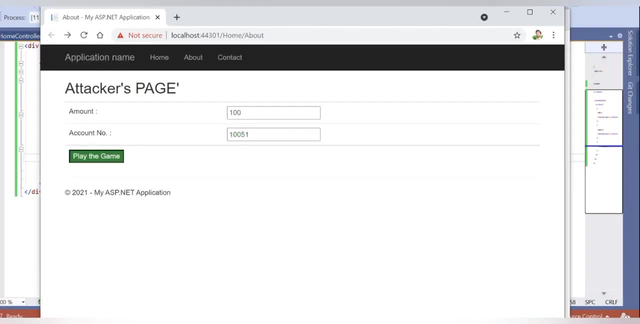 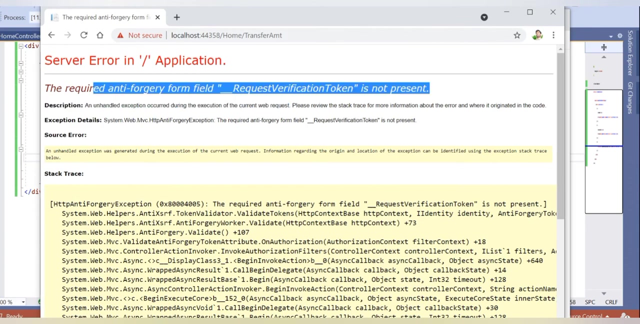 to transfer. okay, this is what going, fine, but now, uh, let's. this is the hacker site, right attackers page. so let's play the game now. now we can see the required anti-forgery from field required verification token. it is because of that, if you will see uh here. 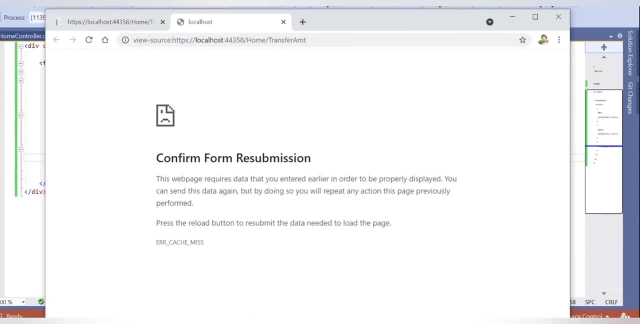 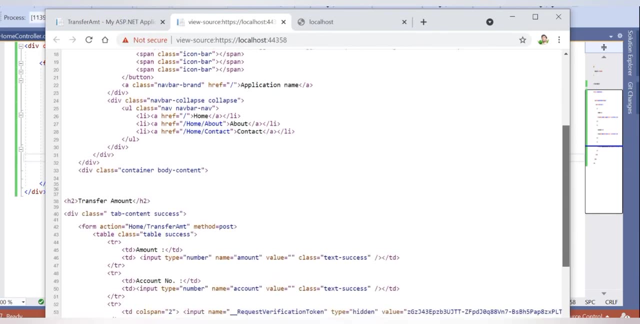 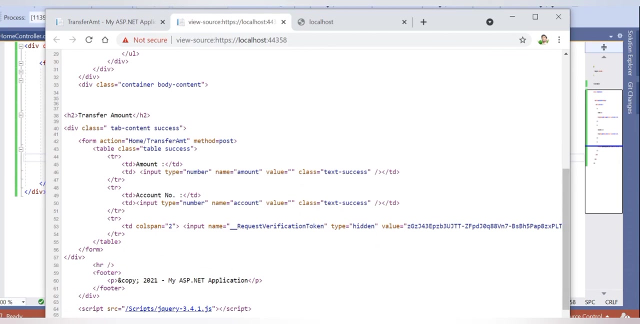 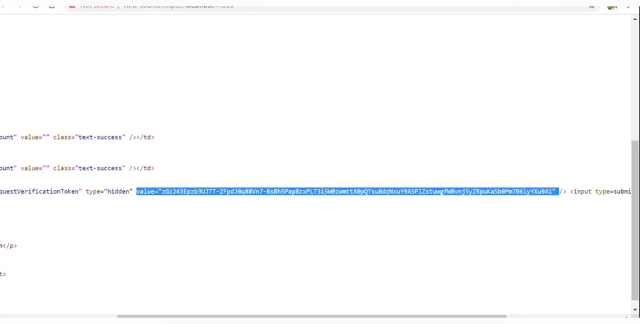 in the view page source. so let's do it back, okay, and view page source. so what is it is doing in case of the uh anti-forgery token? that's, it is creating the uh cookies here. see, it is creating the cookies here, this cookies it is creating. so it now it can be accessible on the same page, in which.